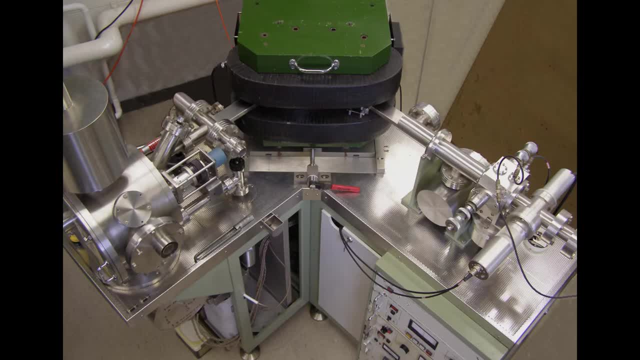 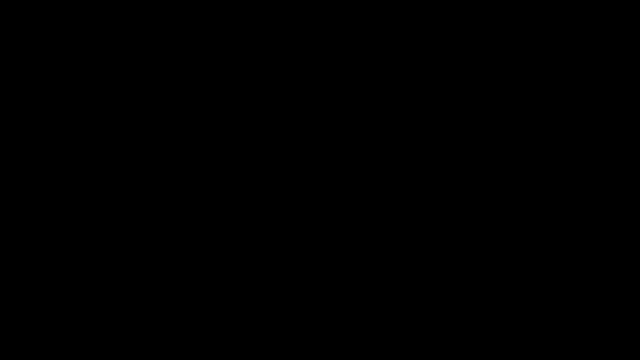 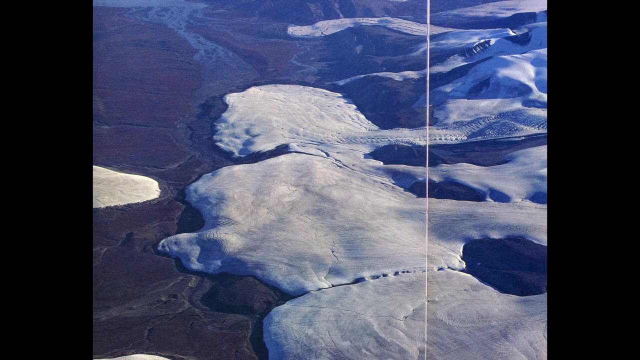 constrain the timing of recent glacial events. We're talking about last 40,000 years. Although this technique depends on location, suitable organic material, It's not always correct, but still, scientists date a lot of deposits, cross checking, cross correlating, and we have 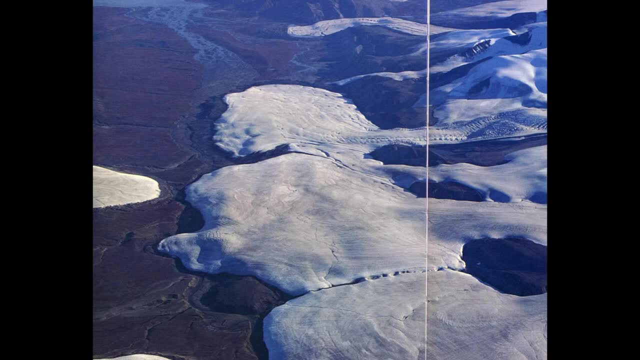 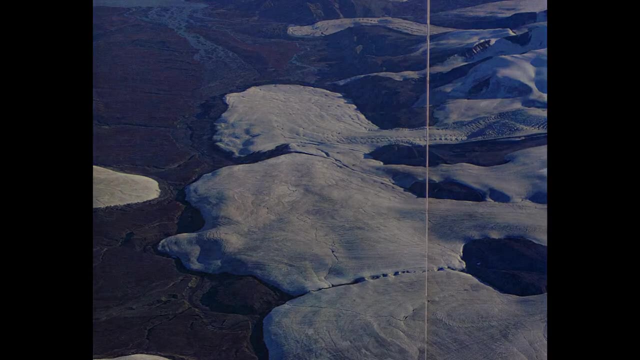 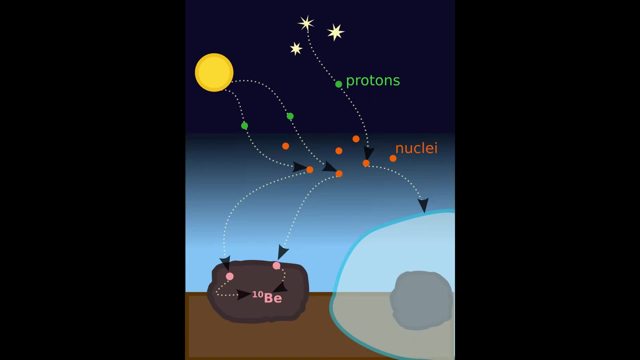 more or less approximate dates for particular deposits. These chronologies have been revolutionized in the first decades of the 20th century also by new cosmogenic radionuclide methods And also optically stimulated luminescence dating. These techniques date the duration of the 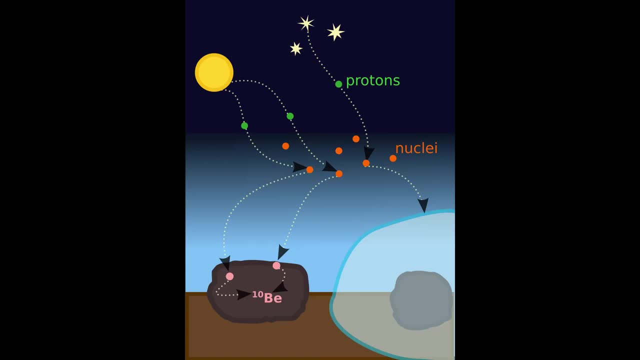 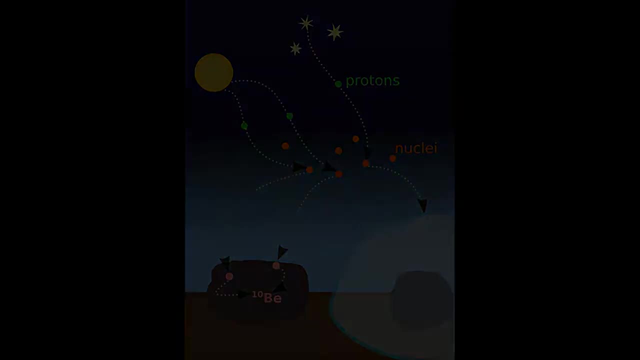 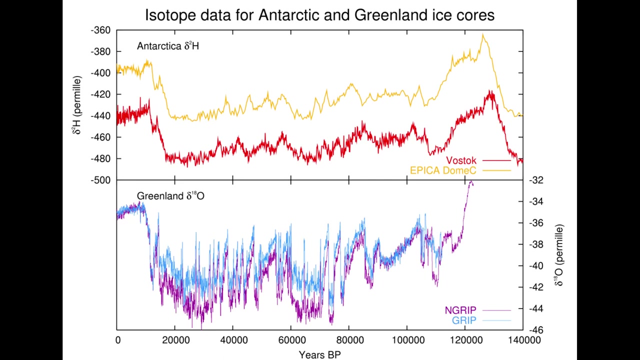 surface exposure in the age of sediment burial and allow us to place glacial chronologies on the absolute time scale, and we can correlate it with other data from marine and ice core records. Thus, today we have quite secure data from particular oxygen isotope ratios in marine sediments. 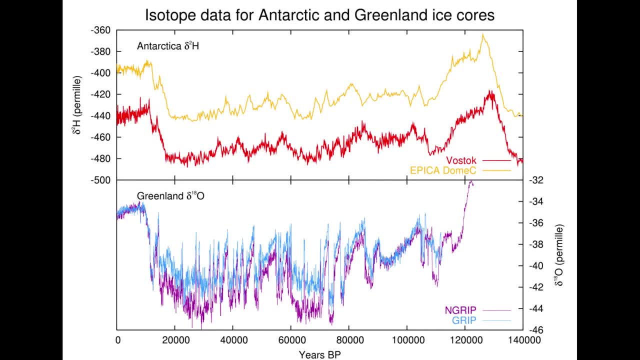 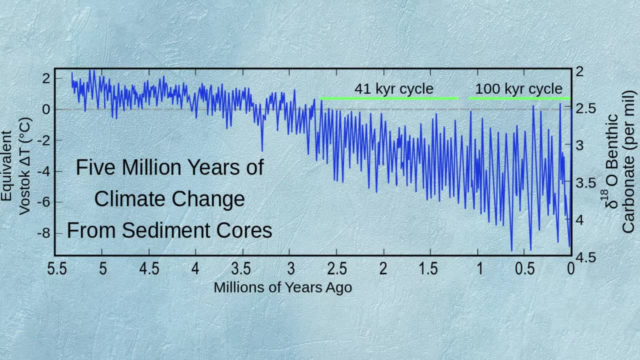 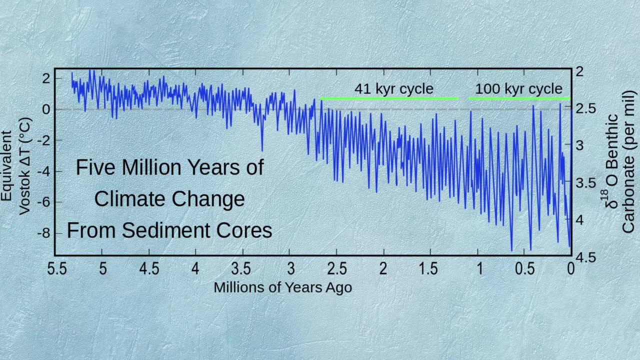 and also from the ice cores in Antarctica and Greenland Marine isotopes record provide a benchmark chronology for the quaternary period. Thus we can kind of look in the last two million years or so up to present time and see quite detailed record of fluctuation of those isotopes. 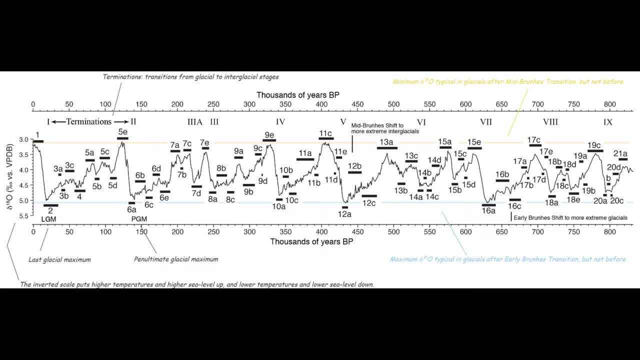 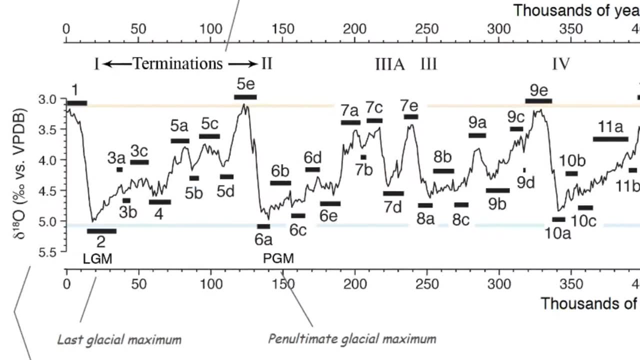 Thus this marine isotope stages we called MIS number back from the present till past, With cold periods assigned to even numbers and warm periods to odd numbers. The current warm period is assigned to be MIS 1 and the last period when there was a cool event. 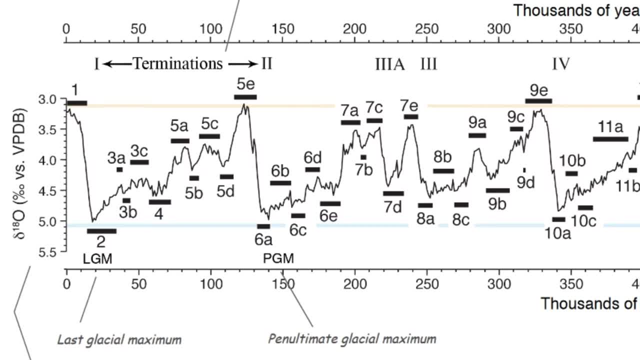 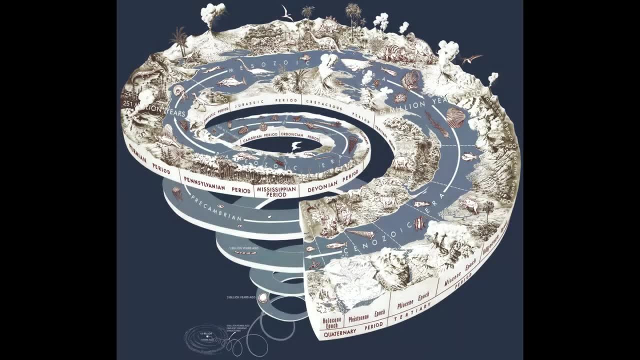 full glacier conditions. we called MIS 2 or last glacial maximum. All these periods characterized by glaciation, but the location or extent of the ice sheets will vary When these correlate these changes. since the onset of the ice sheet glaciation in the early 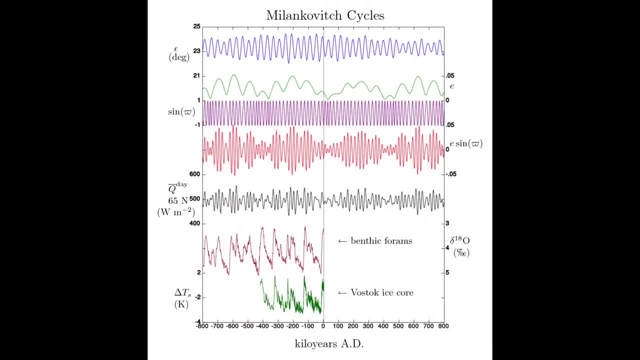 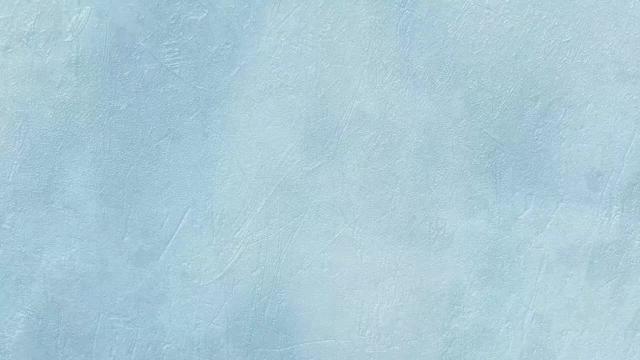 Yggdrasil to the obliquities cycles about 40,000 years. Watch my video about the Milankovitch cycles. Around 800 to 900 thousand years ago, the dominant wellness of climate cycles switched to approximately 100,000 years, close to eccentricity cycles. 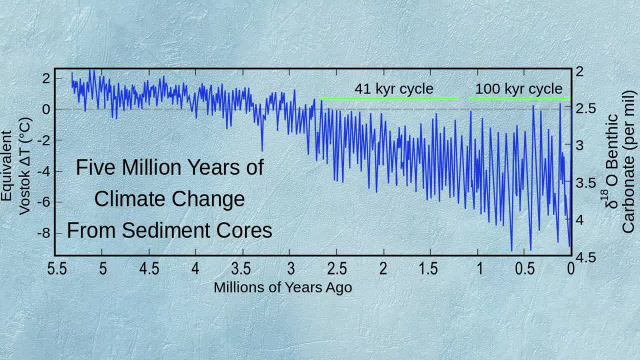 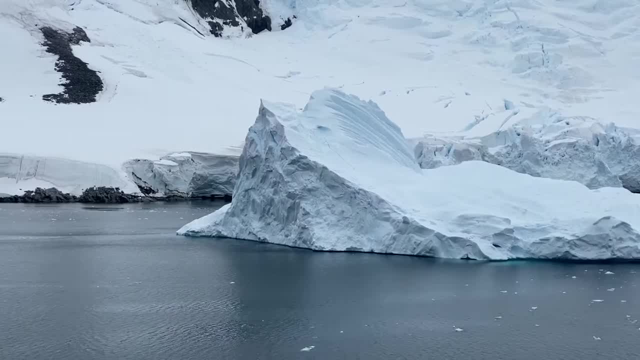 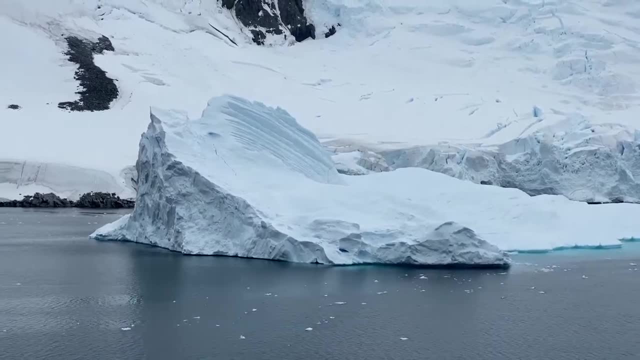 Scientists argued why one cycle is more dominant than the other, in particular time, And many scientists suggested that it's not a straightforward correlation between the cycles and the climate response on the planet. So it's more non-linear dependencies in the earth system reacting to these changes in our astronomical cycles. 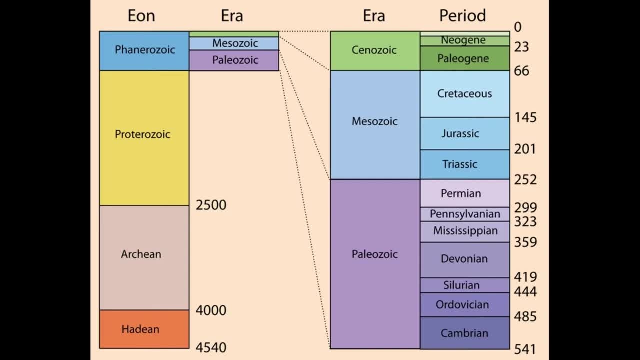 Thus we can say that late Cenozoic glaciations began early in Antarctica. Scientists suggested that Antarctica was under the ice throughout the Cenozoic period, and the ice sheet started growing after the Eocene-Oligocene boundary about 34 million years ago. 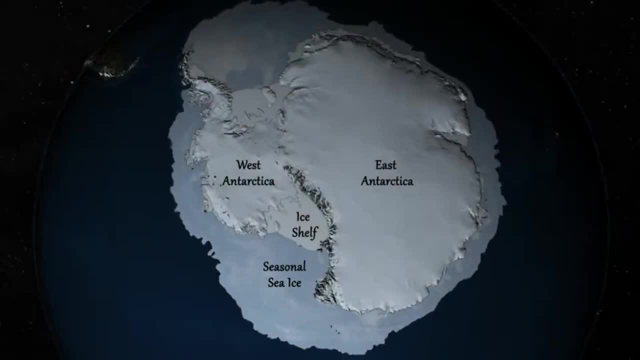 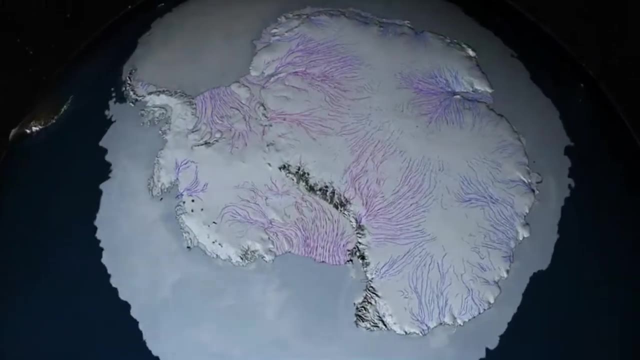 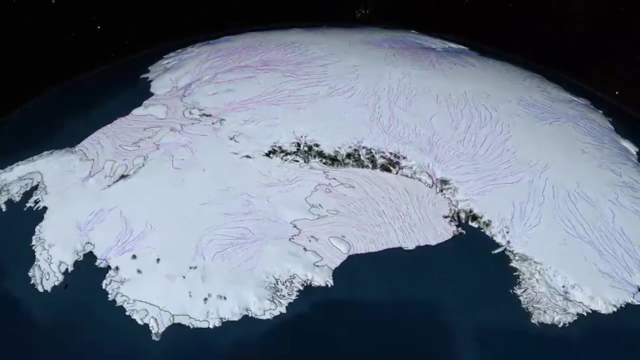 Antarctic ice sheet extended and retreated several times until the middle Miocene climate optimum at about 14 to 10 million years ago, And after that the ice sheet became permanent around Antarctica and that's we're observing today. During the LGM, the last glacial maximum which happened according to the old data on our 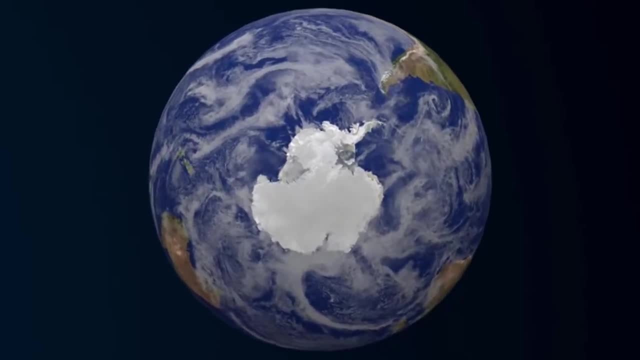 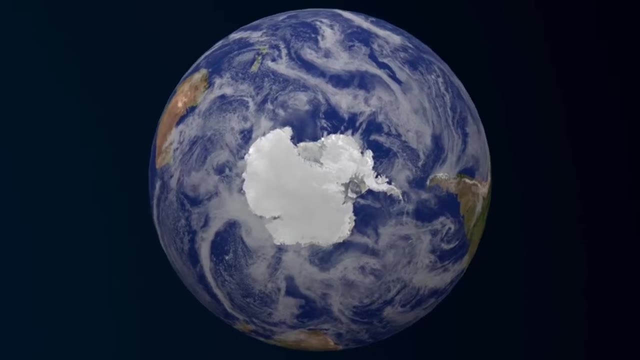 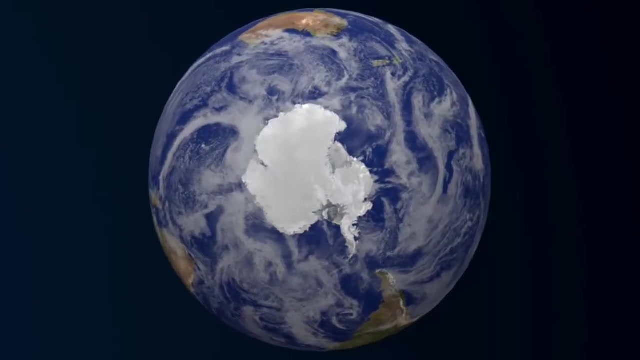 planet about 20 southern years ago. the ice is extended close to the edge of the continental shelf since then. we can note that Antarctica ice sheet right now melting down and some ice start retreating up into the valleys, into the middle of the continent. similar we can observe 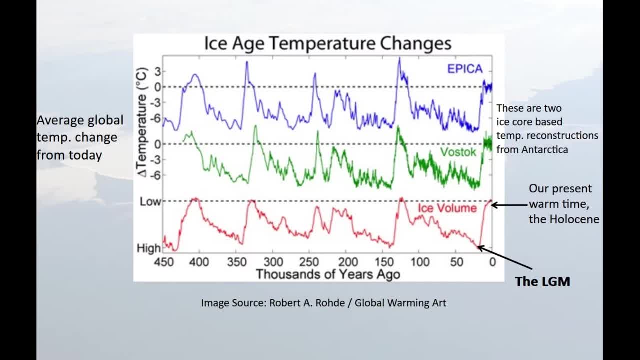 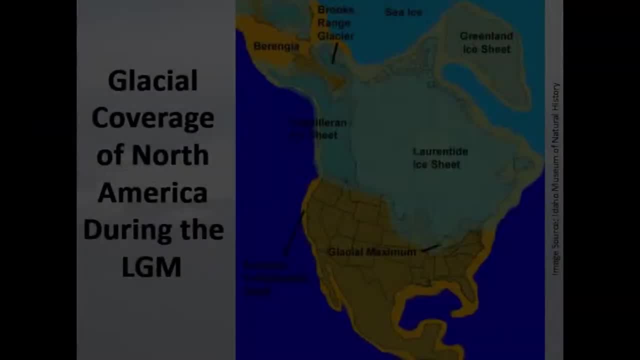 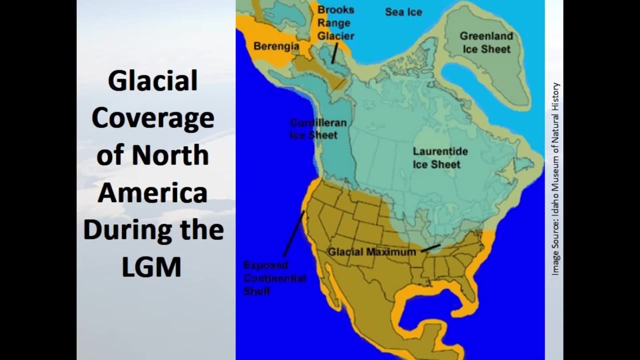 around the northern hemisphere. however, the recent data show that the northern hemisphere glaciation started about 3.2 million years ago. The largest sheet around northern hemisphere is Laurentian ice sheet, which is maximum extent covered large parts of northern North America At the glacial maximum. the Laurentian ice sheet. 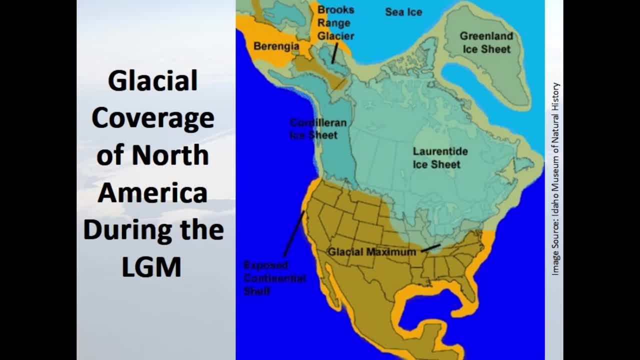 confluent with the Calderian ice sheet at the west of the North America and the Enutian ice sheet in the north. When the cold periods are less extended, less severe, those sheets are separated and behave independently. During the last glacial maximum, which we find out was about 20, 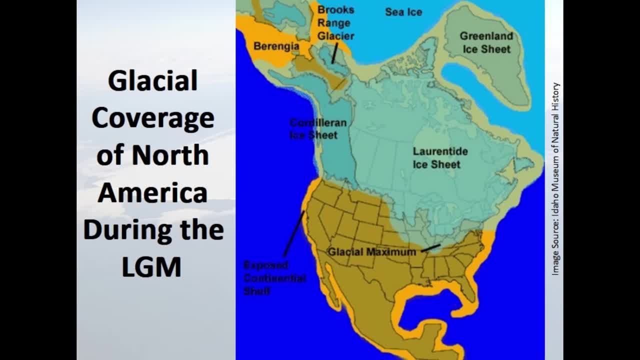 southern years ago. the peak of it, Cú le, keeps observe and exist for 600 thirty adapted Calderán ice sheet extended from the Puget lowlands in Washington state to the western tip of the Alothese Islands. At this time, the inlet sheet covering the Canadian arctic archipelago. 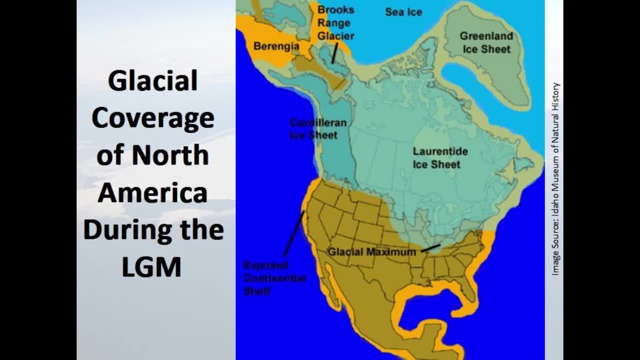 and was composed of the open sector to the east and lowland sector to the west. the ground ice sheet covered the SIBEGAL, Team해주 to the Eesst and lowland sector to the west. The Greenland ice sheet also expanded over the 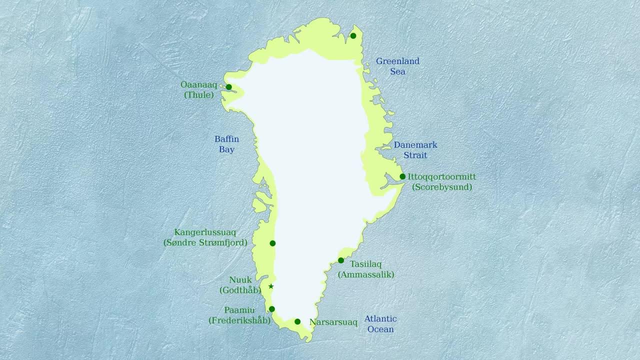 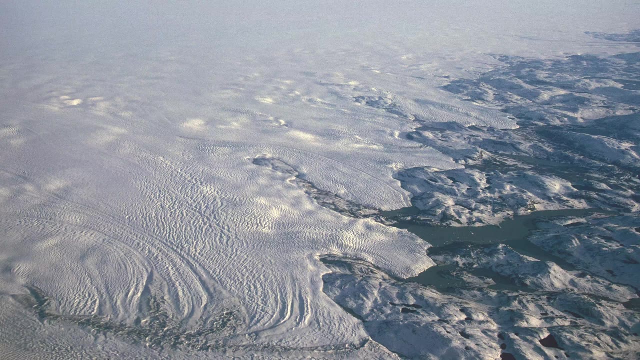 surrounding continental ice sheet, Esmeralda Conva, Argentina, and Shark Tankans, orày Perry, Keeler continental shelf during the LGM or last glacial period, but unlike the North American ice sheets, it's preserved throughout some, but perhaps not all, interglacial periods. We have some evidence that. 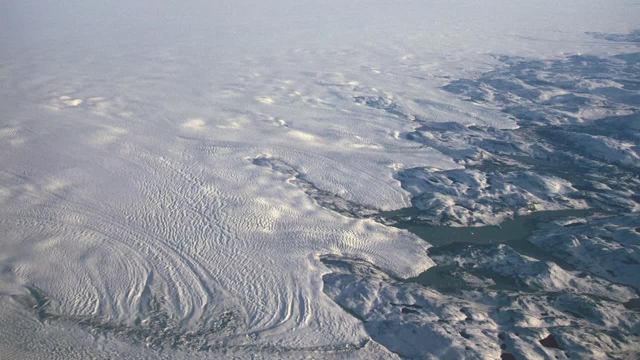 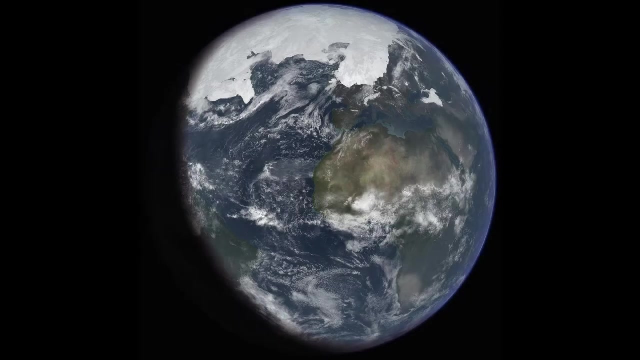 Greenland ice sheet was the smallest in the last interglacial period about 125 thousand years ago, and there was much less ice there than at the present moment. Similar like 20 thousand years ago in the LGM, last glacial period, large ice sheet developed over the Eurasia on several occasion. 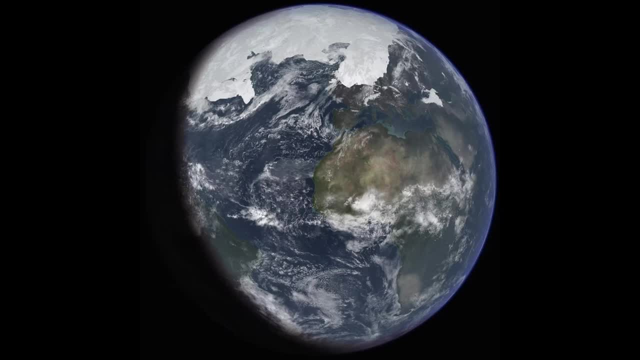 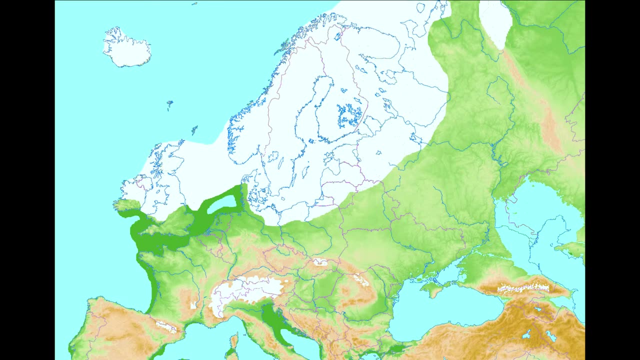 during the last several million years At the maximum extent, Eurasian ice sheet extended from Ireland in the west to Novoe Zemlya in the east and Svalbard in the north Southern areas. margins lay through England, Netherlands, Denmark, Northern Germany, Poland and Russia Northern parts of this. 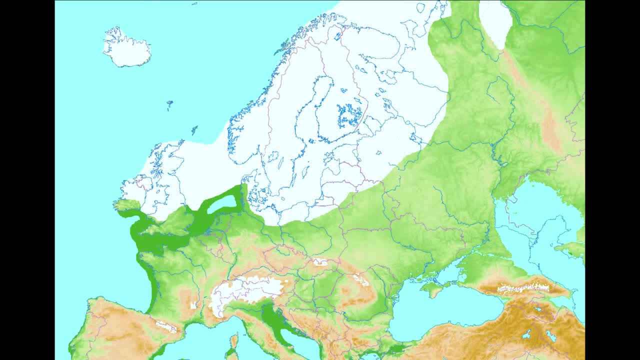 ice sheet grew down to the North American ice sheet and then to the North American ice sheet At the end of the LGM, last glacial period. Greenland ice sheet grew down below the modern level of the sea in the Barents and Clara Seas. It was kind of similar to the present with Antarctica ice sheet. 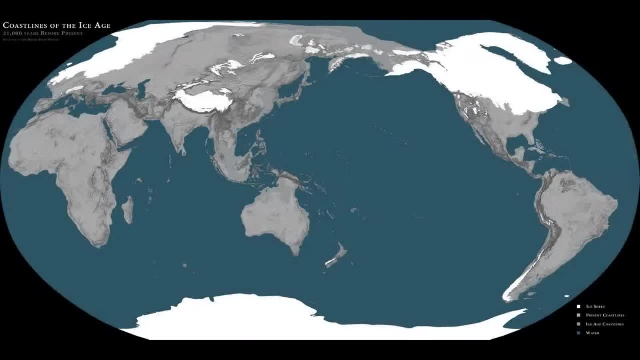 You can imagine that the periods when we have a last glacier maximum, that's, the periods when the sea level is the lowest, because majority of the water being trapped as ice on ice peaks. Therefore, it explains how ice sheets can go further down to the continental shelf outside. 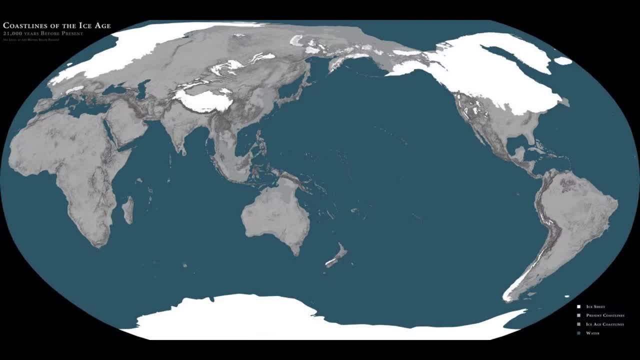 of the modern margins of the ocean. This means that the ice sheets can go further down to the continental shelf outside of the modern margins of the ocean, Because at that time the ocean was much lower. in many places the continental shelf around the continents was exposed and was connecting the continents. For example, when now we see the 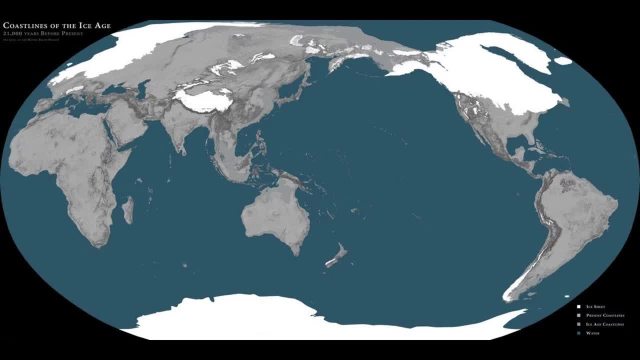 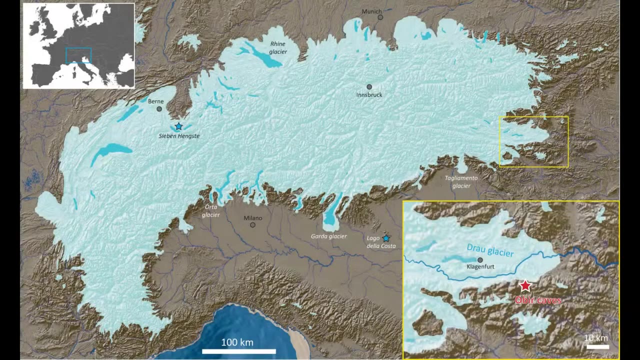 Bering Sea. in the last glacier maximum there was a land connecting North America and Asia, One of the suggestions how the people, first humans, moved from Asia to North and South America. When there was a other glacier maximum periods, the European Alps as well were covered under the 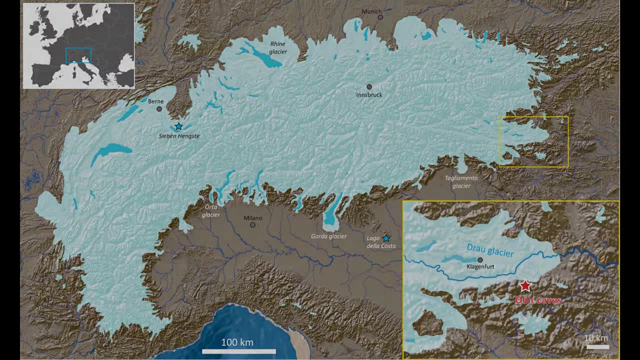 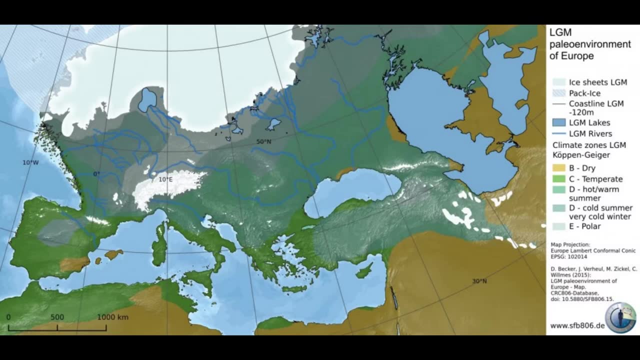 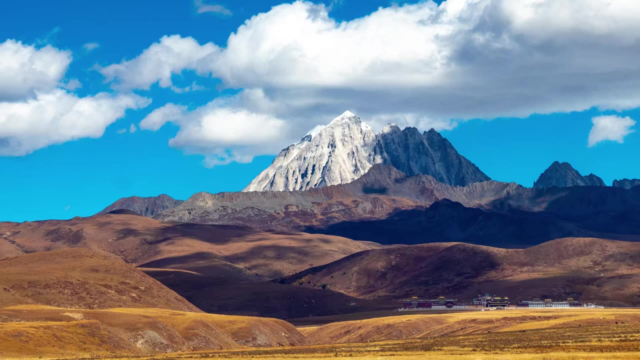 ice and this ice sheet grew further and then it's met the northern ice sheet around the Germany, Poland and they sometime joined together. There's a big ice sheet developed over the Tibet, in the Himalayas, and have a major influence on the global climate. However, some data using the modern technologies of dating suggested that 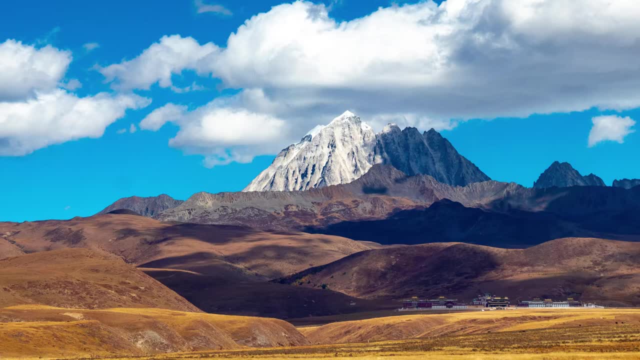 during the last quaternary glaciations. the expansion of the local glaciers in that area in many cases extended only a few kilometers from the present position, And it's demonstrated Tibetan ice sheet have been existed during at least the last few full glacier cycles and kind of in a similar extent as it now. 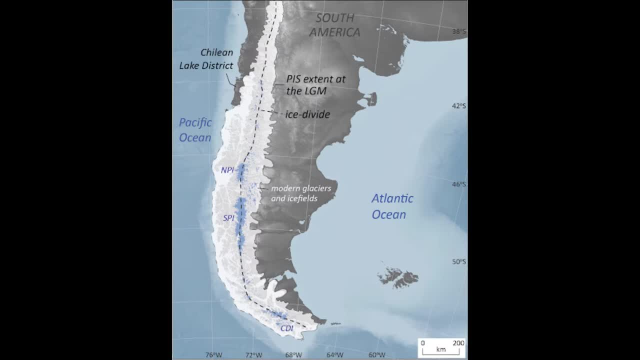 Similar glaciations were observed around South America, Patagonia. there was a big glaciation along Andean Mountains, a developer ice sheet, And the most extensive glaciation occurred in quaternary in southern South America about 1.1 million years ago. We also observed the glaciation. 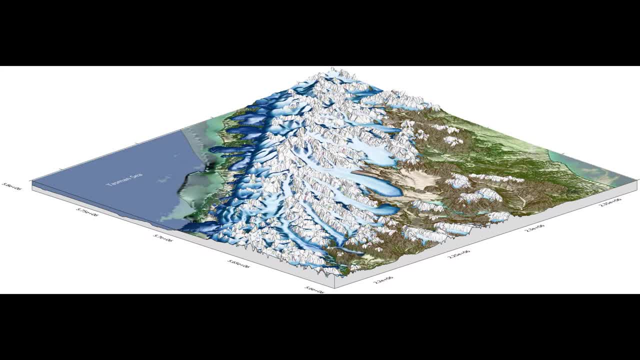 around Southern Alps in New Zealand. We know that still glaciers persist around New Zealand. they're melting away rapidly. However, in LGM those glaciers cover majority of the South Island and the small ice masses develop in places North Island of New Zealand, Tasmania and New Guinea. People finding some evidence of 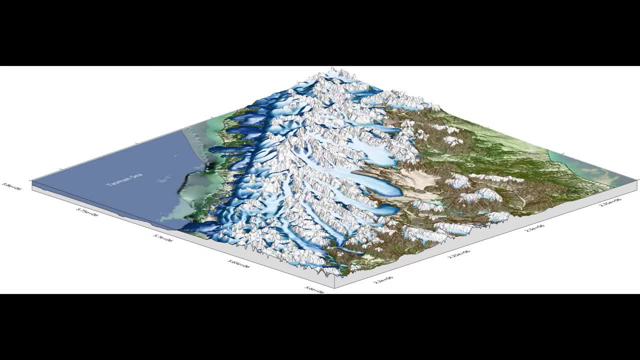 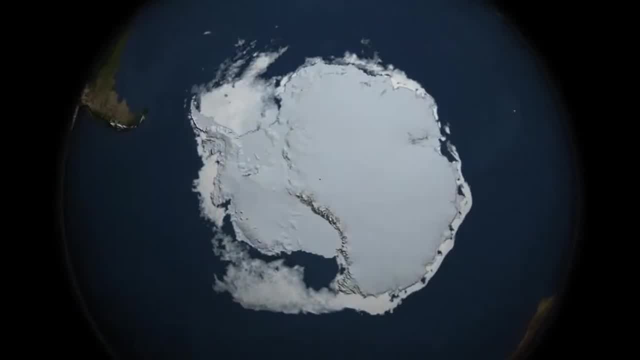 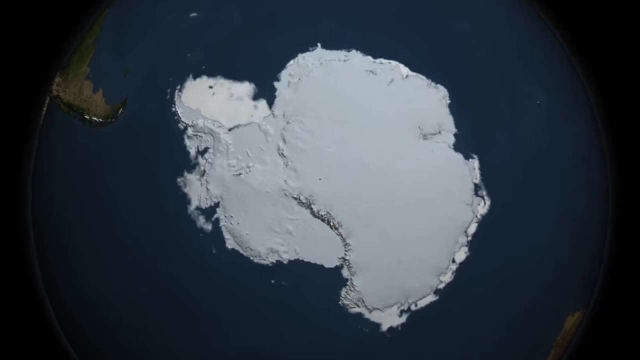 some glaciers even being preserved in LGM around Australia. Therefore, you can see that in the last glacier maximum period, about 20,000 years ago, not only the Europe but also the other parts of the world were affected. Climate on the planet was different and it was not just causing the glaciers going down the valleys. 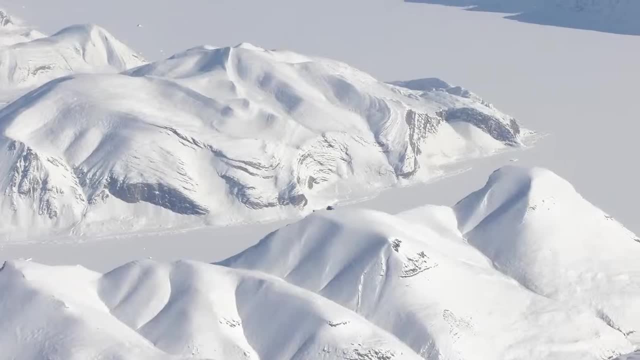 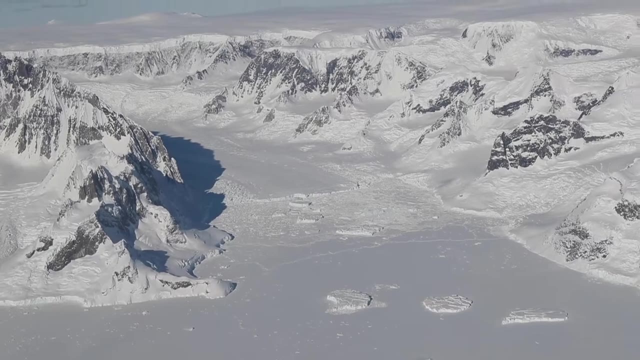 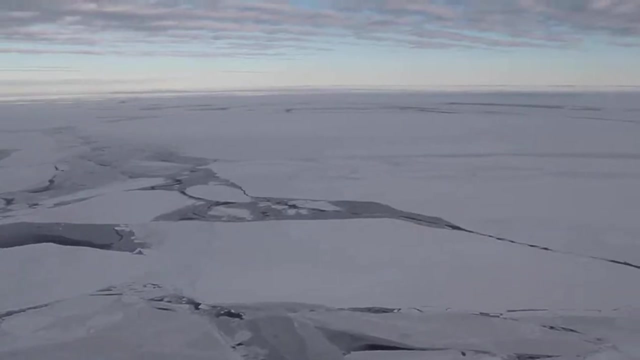 but it's also changing the sea level, changing the vegetation on the planet, forests disappearing, alpine areas increasing cold temperatures around the air become drier, less moisture, and there was a lot of cold winds coming from the big ice sheets down the valleys.